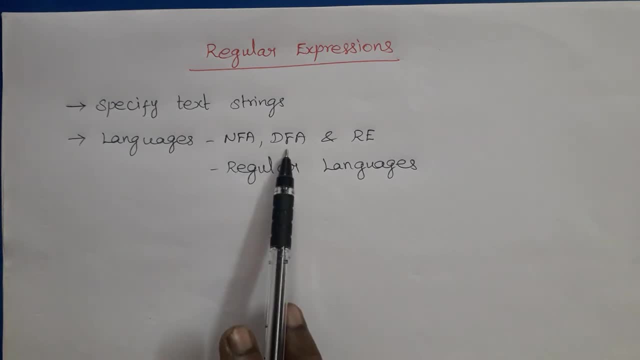 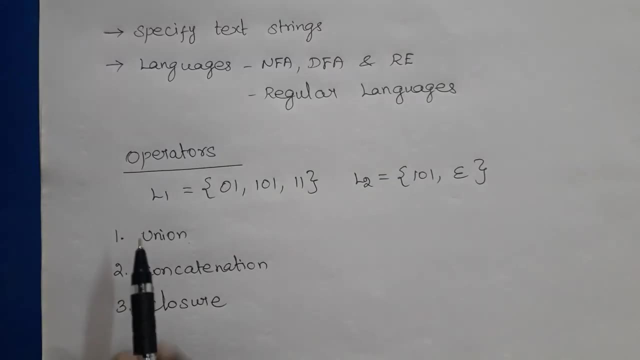 So a language is defined by NFA or DFA, or regular expression is also called as regular language, Then operators can be applied to the regular expressions. First we should know the operators applied to the languages. Assume that L1 and L2 are two languages, So L1 has three strings: 0,, 1,. 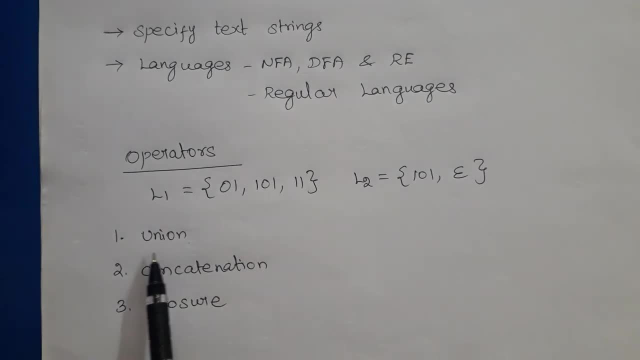 1, 0, 1, 1, 1 and L2 has two strings. There are three operations can be applied to the languages: union, concatenation and, closer So, union of L1 and L2.. This is written as: 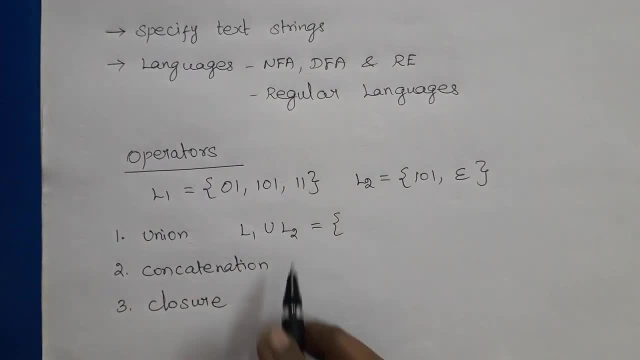 L1 and L2.. So L1 and L2 are two languages. So L1 and L2 are two languages. So L1 and L2 are two L1 and L2.. This language has the set of strings chosen from either L1 or L2, or in both. So it has. 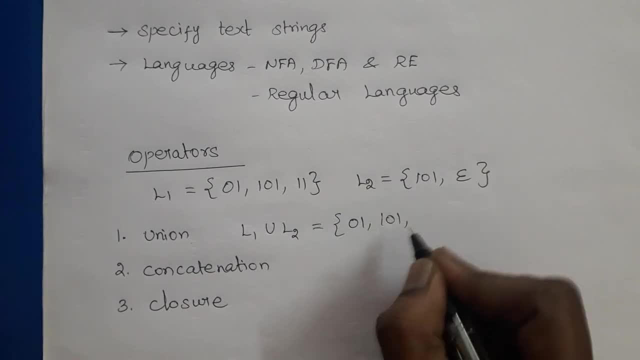 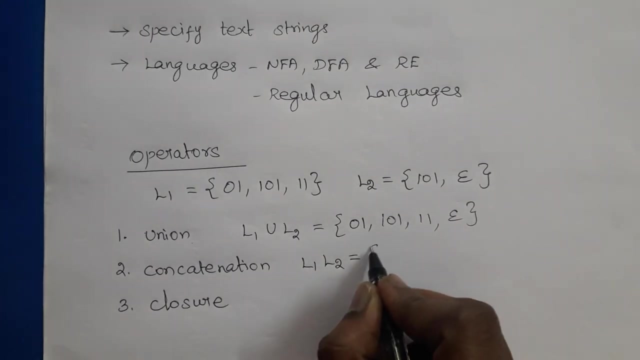 0, 1, 1, 0, 1, 1, 1, 1, 0, 1 is already written, So epsilon. So these are the set of strings in L1, union L2.. Concatenation is written as L1 concatenated with L2.. So here it has the set. 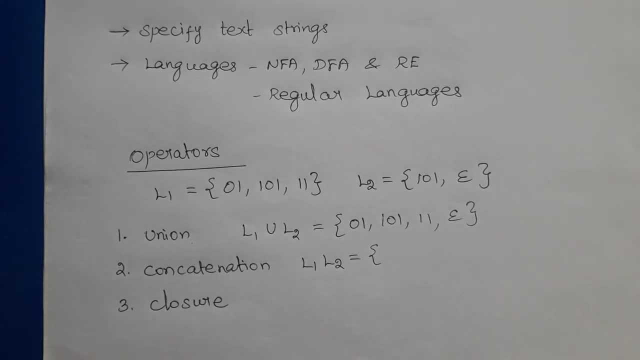 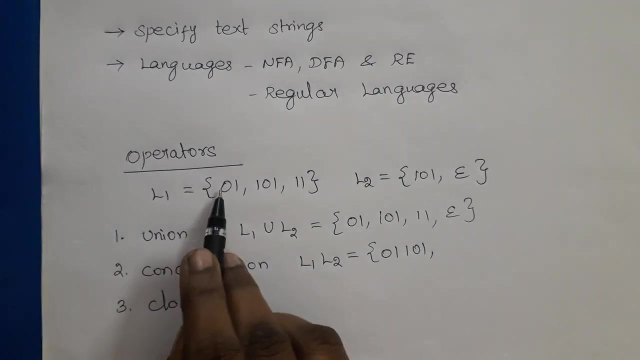 of strings that can be formed by taking the strings in L1 and concatenating it with the strings in L2. So L1L2 equals 0, 1, 1, 0, 1.. Then 0, 1 is concatenated with epsilon. Epsilon is an identity. 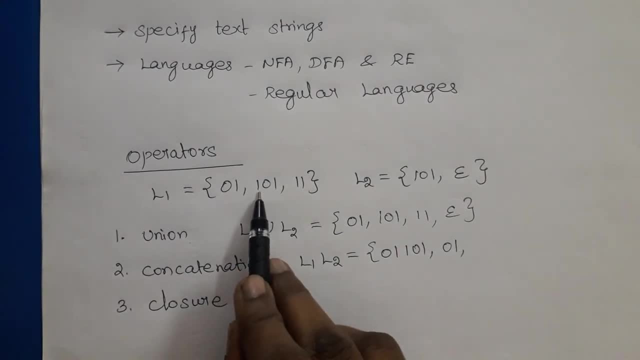 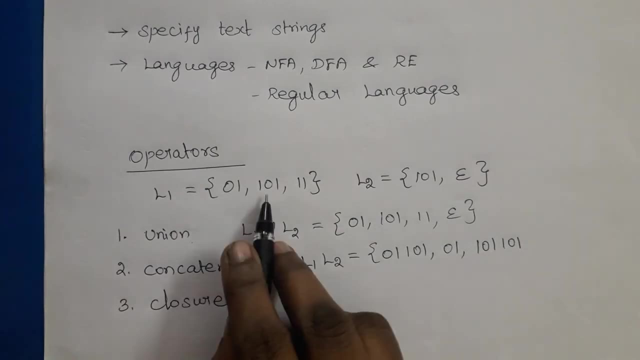 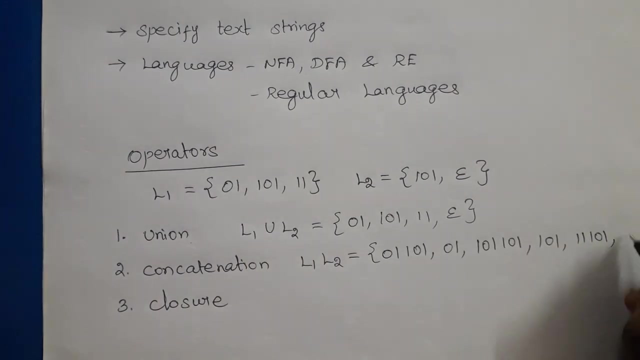 element during concatenation, So 0, 1.. Then take the second string, concatenate it with all the strings of L2.. So 1, 0, 1, 0, 1, 1, 1.. 1 0, 1, then 1, 0, 1 is concatenated with epsilon, then 1 1, 1 0, 1 1, 1. so these are the set of. 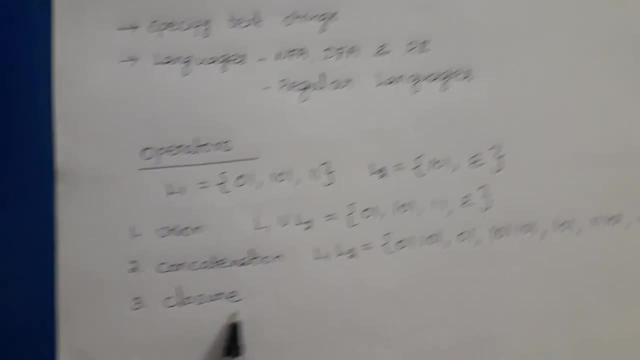 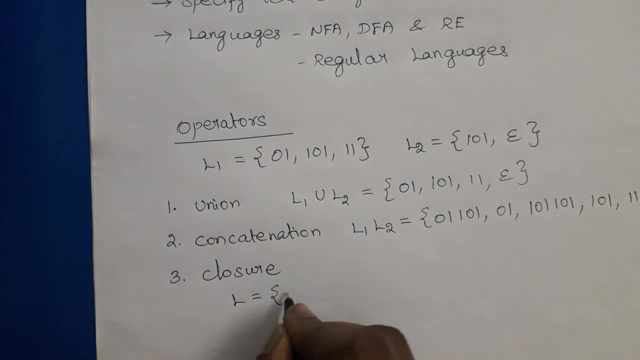 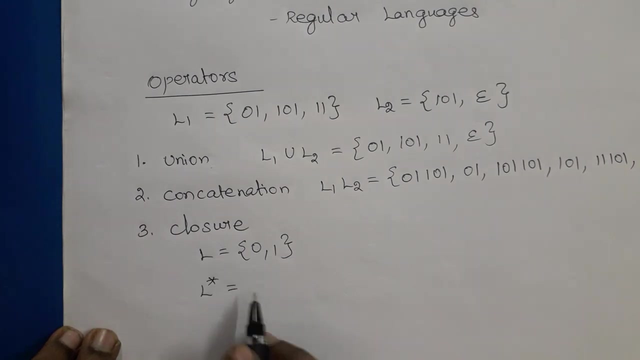 strings in L1 concatenated with L2, then closer operator. this is normally denoted by star: cleanly closer. so if L is equal to 0 comma 1, then L star has the set of strings that are in any string, any combinations of zeros and ones including epsilon. so first epsilon, then if you 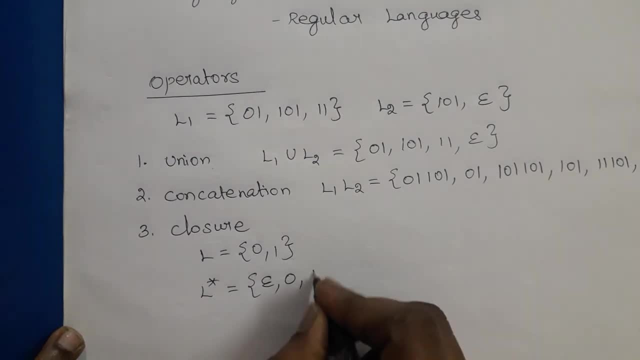 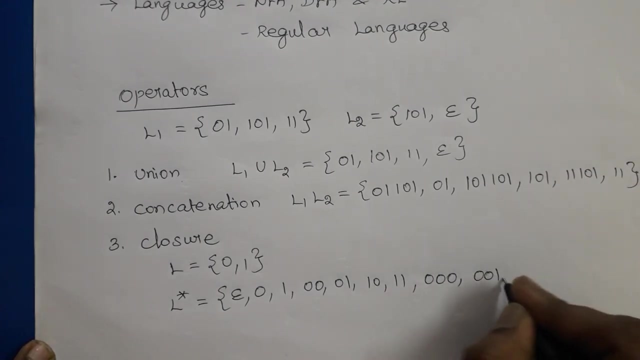 take one string from L, 0 and 1, then if you consider two length string- 0, 0, 0, 1, 1, 0, 1, 1- then 3 length strings can be formed like 0, 0, 0, 0, 0, 1, 0, 1, 0, 0, 1, 1, etc. So set. 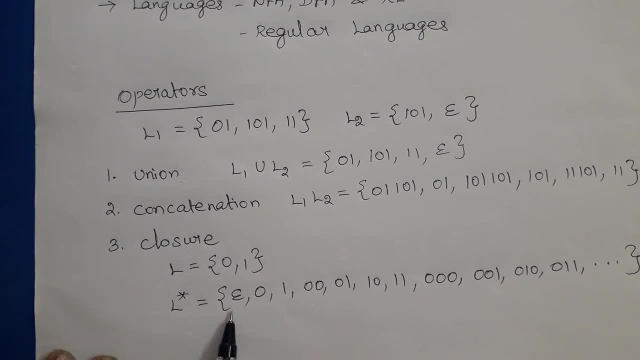 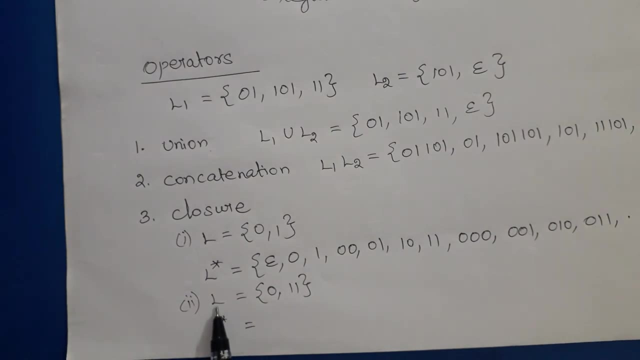 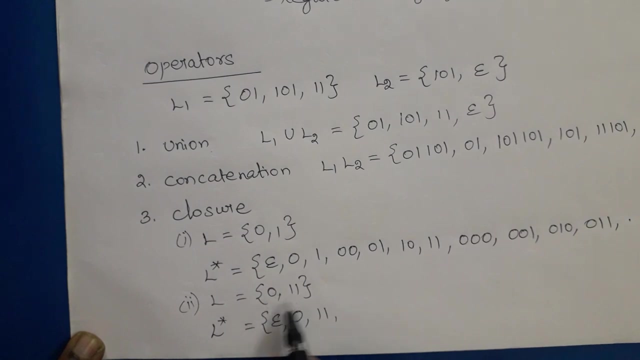 of all combinations of 0s and 1s. this is called as L star. If we consider the second example, if L is equal to 2 strings- 0 and 1- 1, then L star represents epsilon 0 length string. then one time we can choose this string. so 0 and 1- 1. then 2 times means 0, 0, 0 and 1: 1. 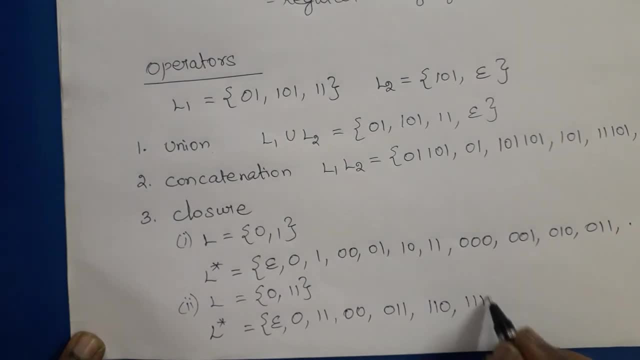 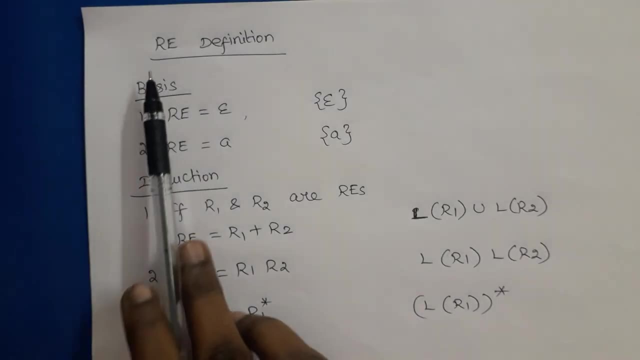 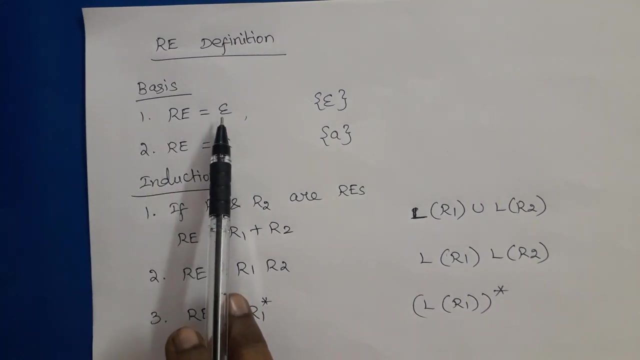 1, 1, 0, 1, 1, 1, 1. so 1, 1 will come in pairs. Now the regular expression definition. there are two basis conditions for any language. regular expression is equal to epsilon. Epsilon is a regular expression denoting the language, epsilon, that is. it is the set containing only. 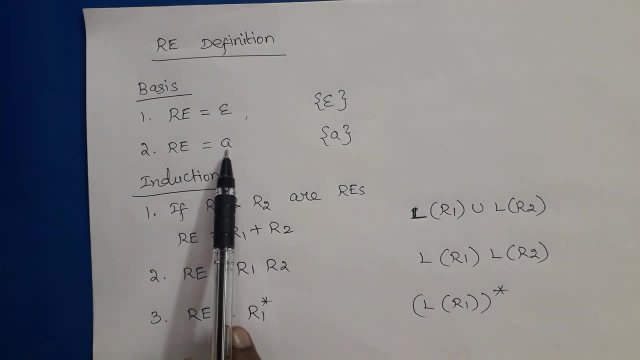 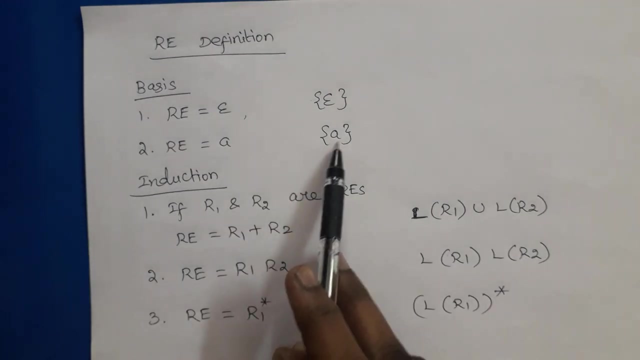 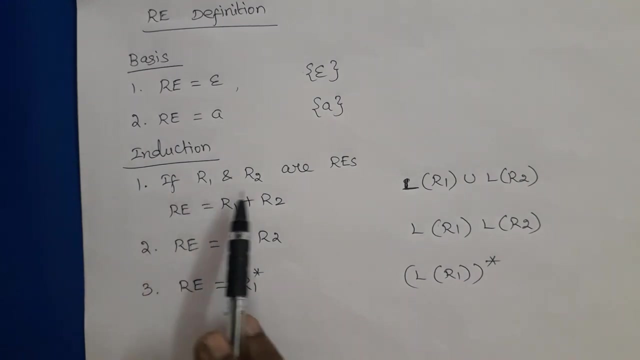 epsilon, then if a is any symbol, it may be a symbol in input alphabet, then a is a regular expression. it is denoting the language containing only a. it can recognize only a then by an induction step. there are three cases. if r1 and r2 are, 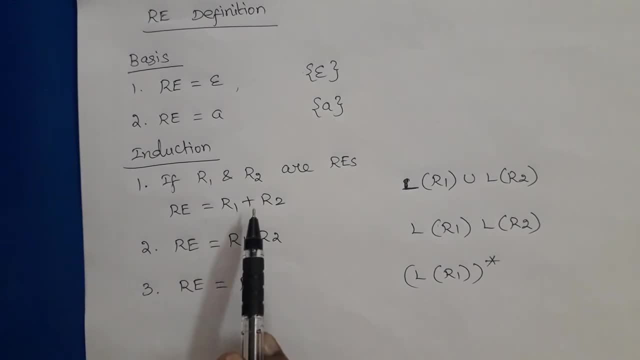 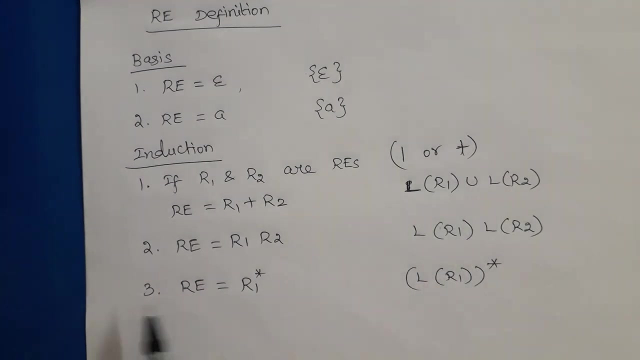 regular expressions. then we can frame: r1, union, r2 plus plus is representing union operation. sometimes a bar is also used, so vertical bar r plus denotes the union operation, so regular expression is equal to r1 plus r2.. usual expression is used to denote the language of l1, union, l2, and in second case we can apply: 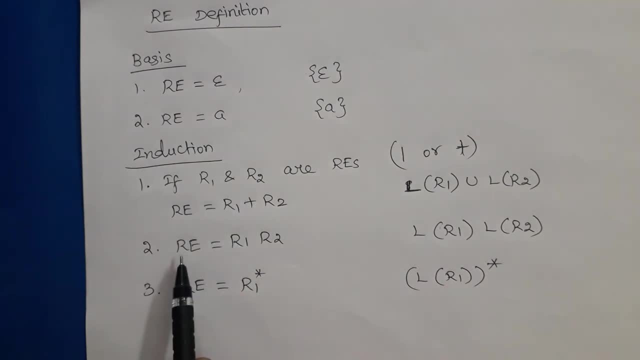 the concatenation to these regular expressions. so we can frame regular expression r1 concatenated with r2.. If r1 and r2 are regular expressions, r1 concatenated with r2 is also a regular expression. It denotes l of r1 concatenated with l of r2. and then if r1 is a regular expression, we 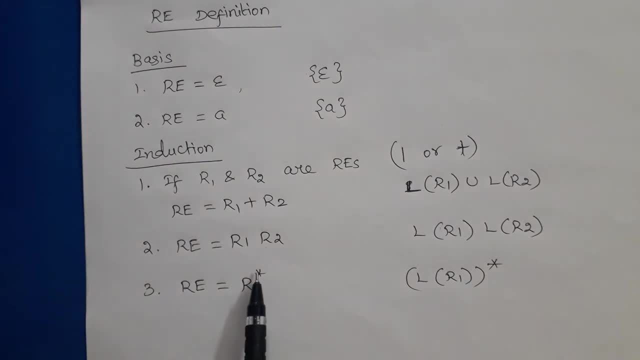 can say that r 1 star is also a regular expression and if it is regular then l of r1 as left, as b as a regular expression can also be terms. So therefore we can say that if r1 star is star Kleene closer is also a regular expression. It is used for denoting the language, L of 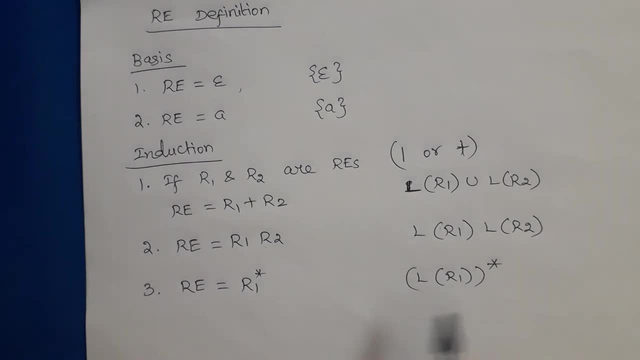 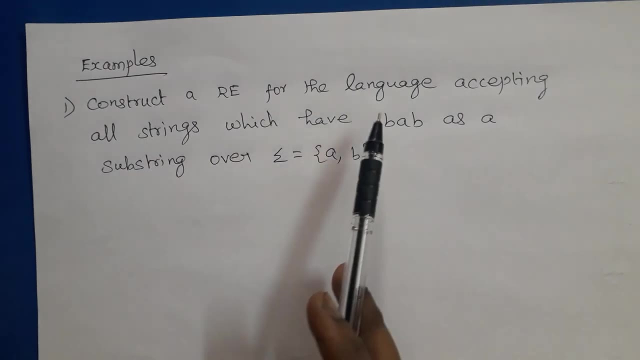 R1 star. It represents 0 or more instances of R1.. Consider an example, That is, we need to construct a regular expression for the language accepting all strings which have B, A, B as a substring over the input alphabet A and B. That is a regular expression, Regular. 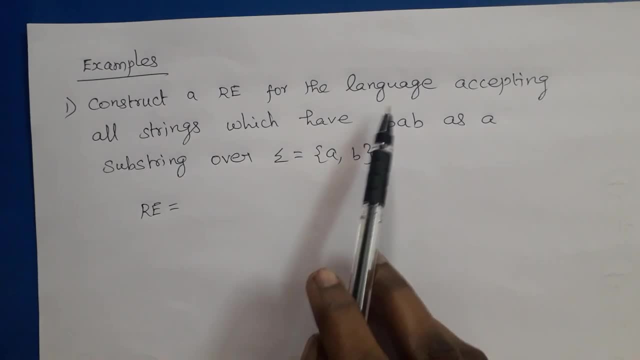 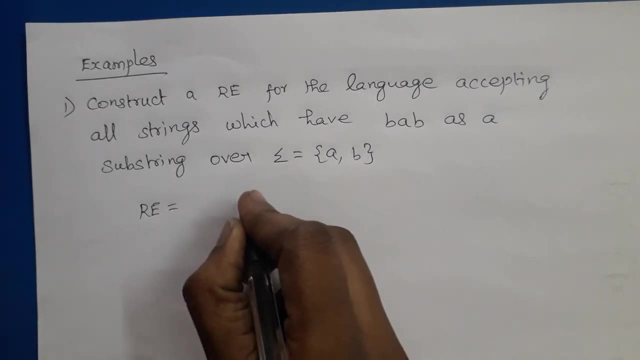 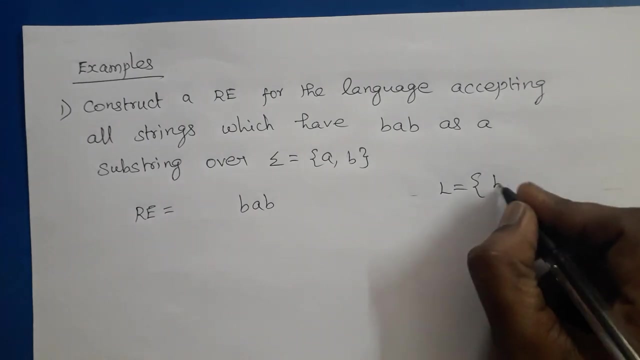 expression is used to denote a language, So the language consisting of a set of strings in which all the strings should have B A B as a substring, So all strings should have B A B, So it can recognize this regular expression, can recognize the language of strings. 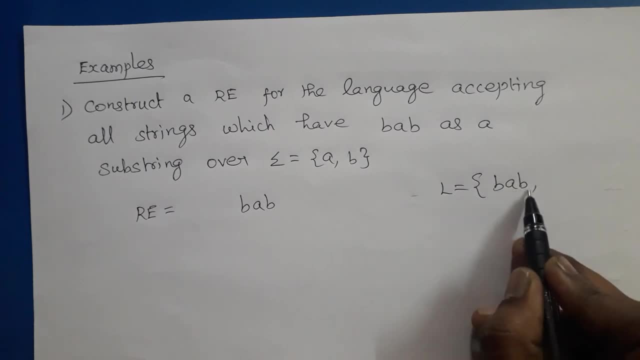 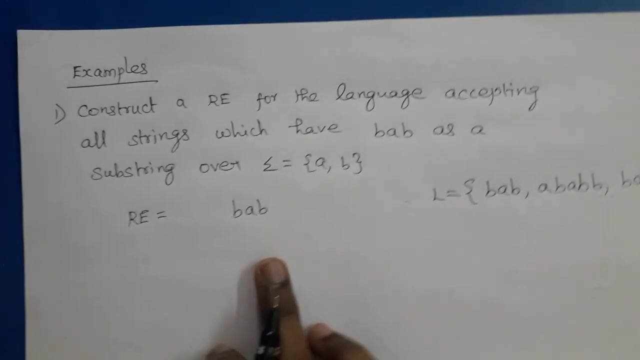 B A B, because this string has B A B as a substring, or B A B preceded by A, followed by some B B A. So these types of strings must be accepted by our regular expression. So you regular. 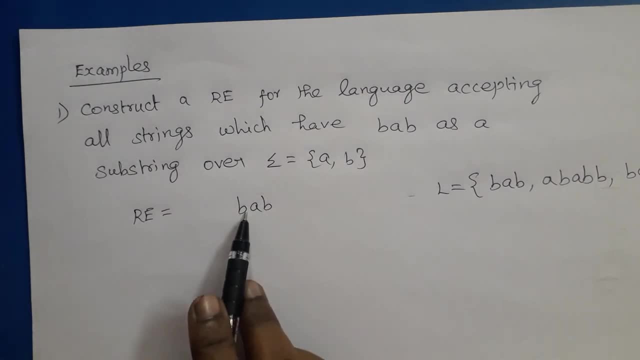 expression equals B, A, B, and this sequence should be preceded by any number of A's and B's, So any number of A's and B's means we can write A plus B star Or A vertical bar B. star represents any number of a's and b's. a plus b means a union, b, a or b, so star represents. 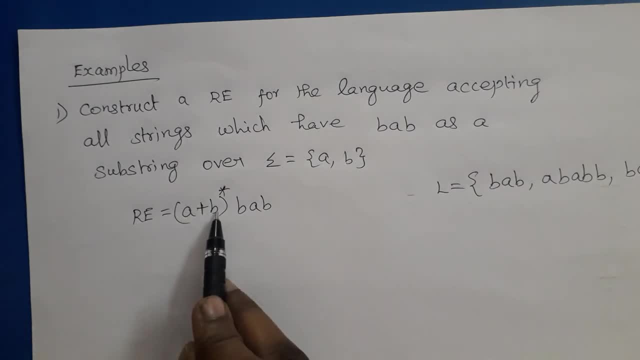 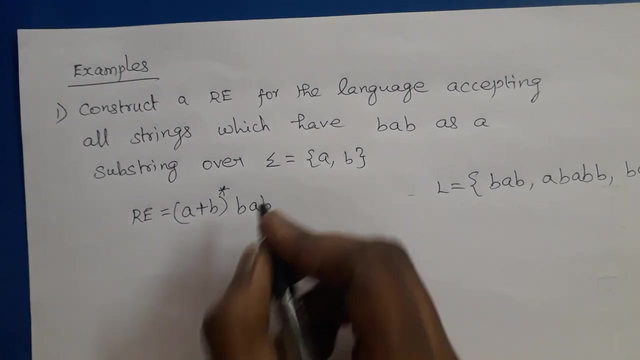 zero or more instances of a and b, any combinations of a and b. so this b a b can be preceded by epsilon. also because b a b is a correct input string. so b a b is preceded by a plus b whole to the power star and should follow, followed by a plus b star. so this is the regular expression.